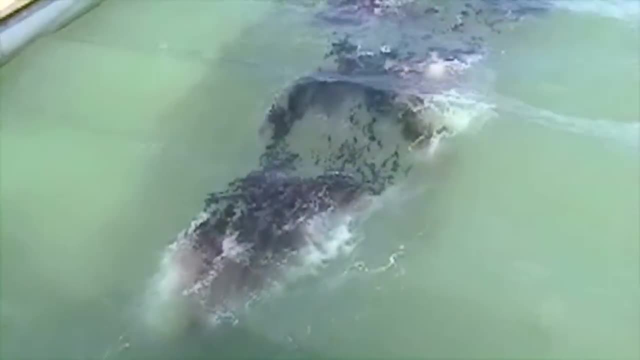 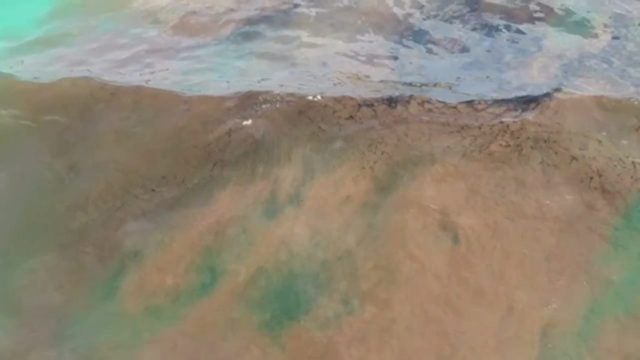 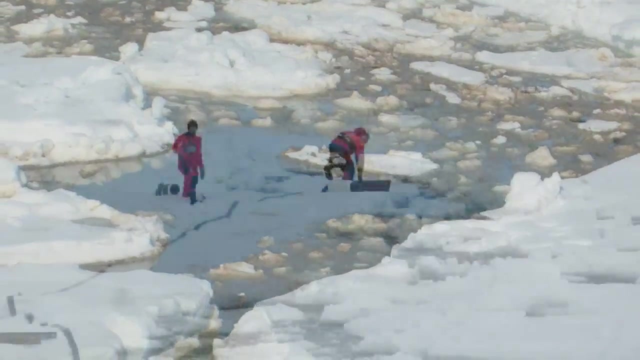 which occurs even at low temperatures. This biodegradation can be aided by chemicals called dispersants that break down oil into smaller particles. However, more research is needed to determine the fate and effects of chemically dispersed oil in the Arctic environment. Responders often burn oil where it is spilled. 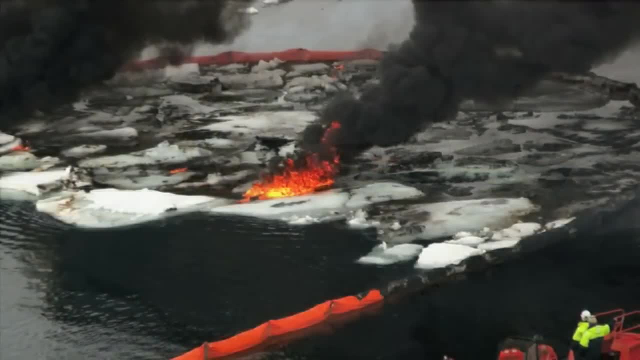 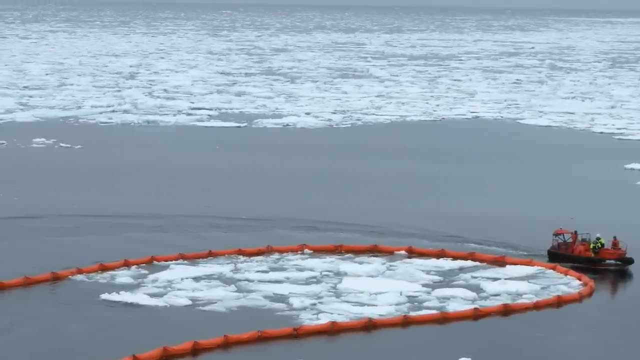 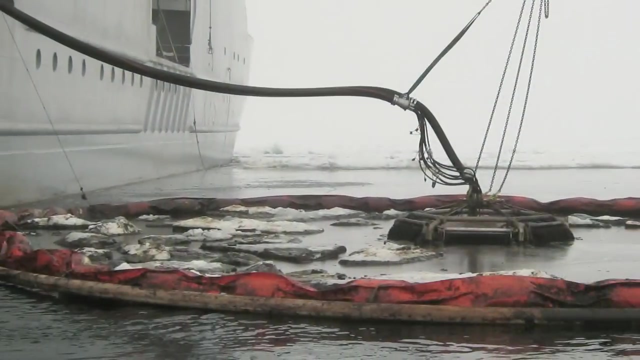 This: in situ burning can be very effective in Arctic conditions, as sea ice can help collect oil and thicken oil slicks, But in open water oil will quickly spread too thin for ignition. The mechanical recovery of oil using booms and skimmers to contain oil slicks. 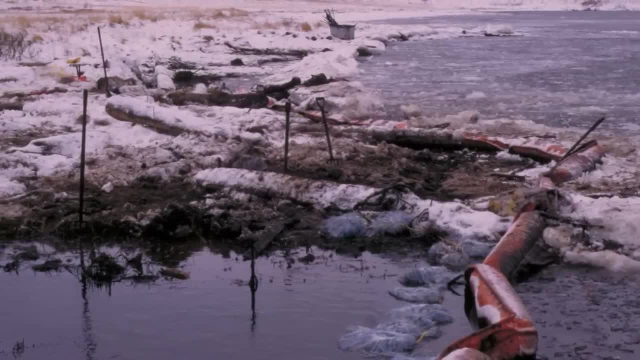 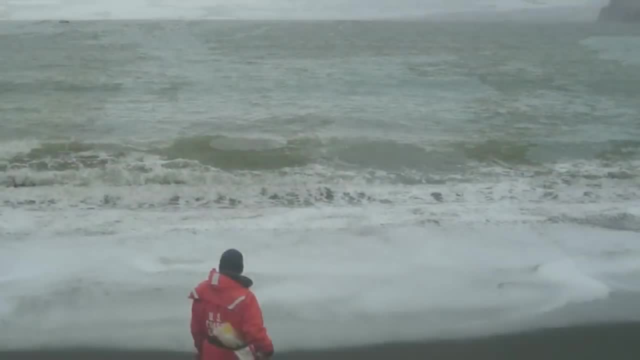 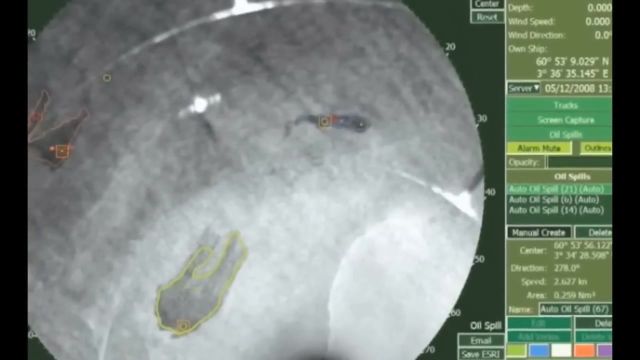 will be difficult in Arctic conditions, with difficulty in deploying resources to remote areas, few approved disposal sites for contaminated waste, poor port facilities for vessels and limited airlift capabilities. Knowing the location of spilled oil is critical to mounting an effective response. Over the past decade, advances have been made in detecting and modeling oil. 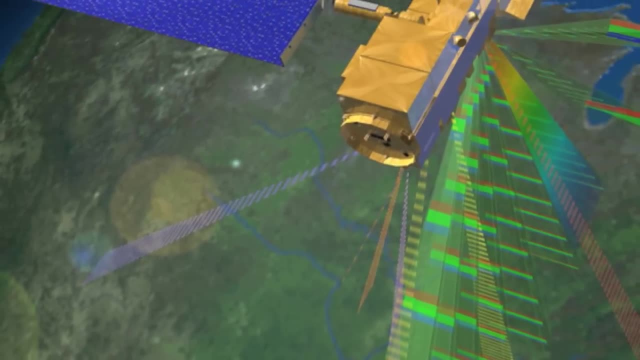 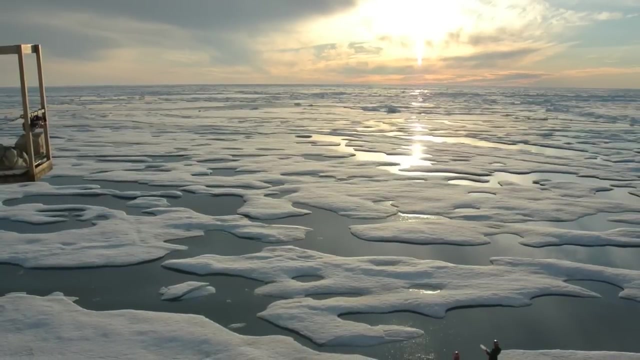 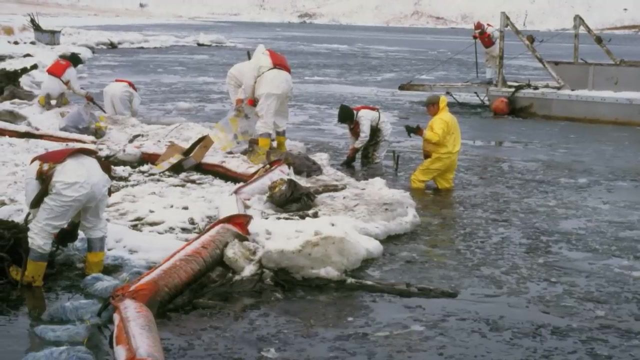 on and under ice, using remote sensing technologies and autonomous underwater vehicles. The Arctic is remote, geographically vast and lacking in the infrastructure needed for oil spill response, presenting a significant liability in the event of a large oil spill. Pre-positioning response equipment. 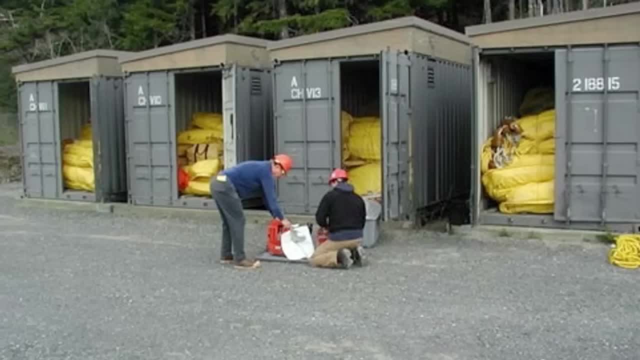 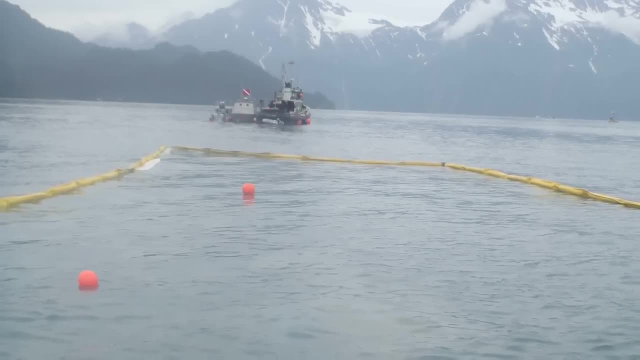 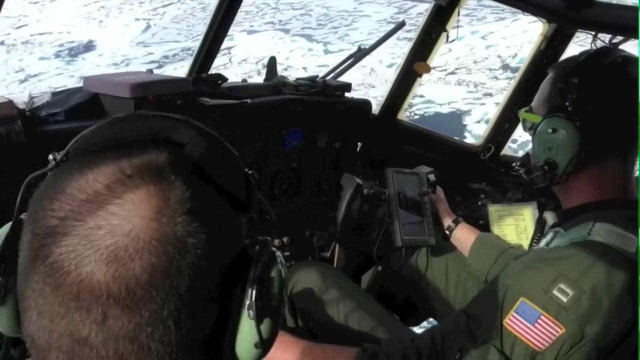 such as in situ burn materials or dispersants at strategic locations, would help provide faster response, as would enhancing the presence of the US Coast Guard in the Arctic. There is no one-size-fits-all strategy for Arctic oil spill response. Instead, research is needed to build a toolbox. 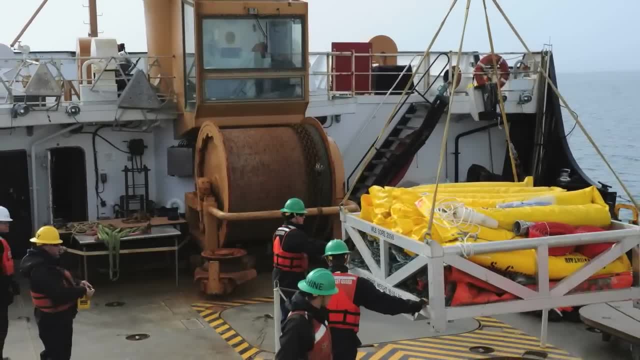 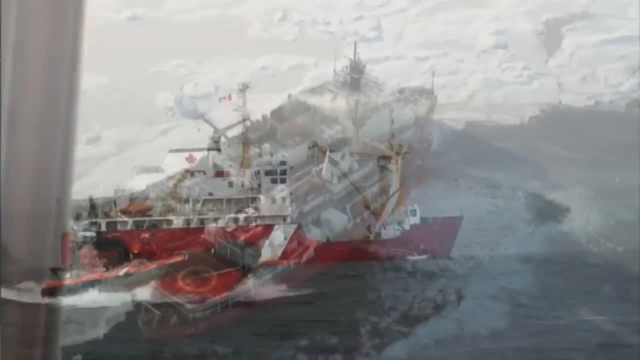 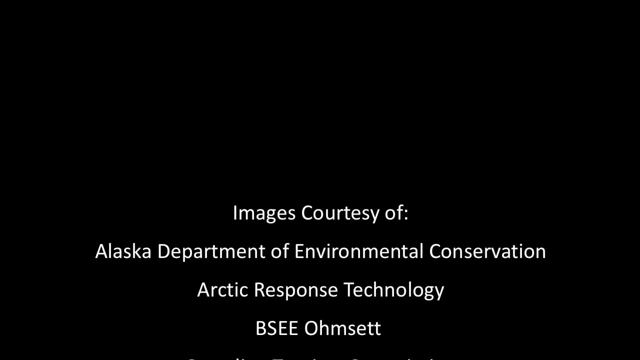 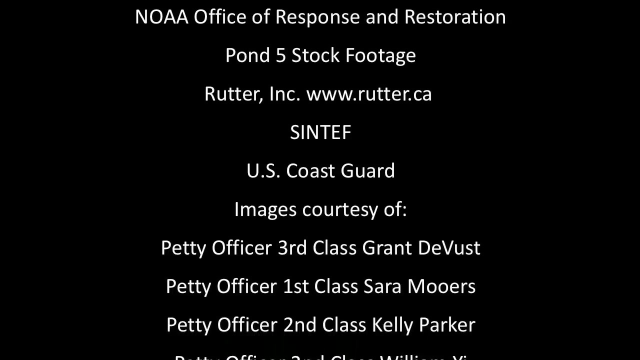 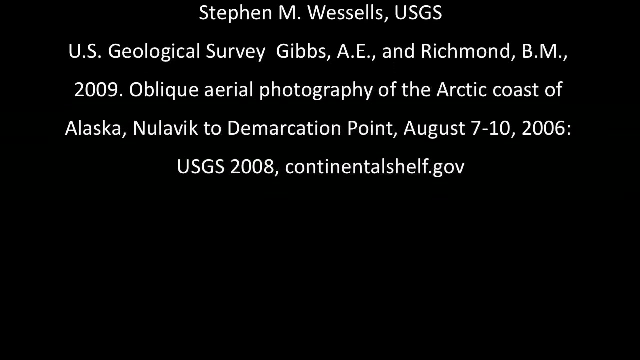 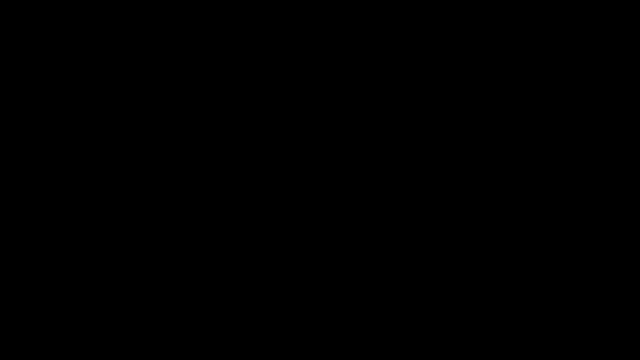 of proven Arctic oil spill response technologies that together provide the flexibility needed to mount an effective recovery effort in challenging conditions. The Arctic Ocean Council has been working closely with US Coast Guard to evaluate, develop and implementleri in the Arctic region. NASA Jet Propulsion Laboratory, California Institute of Technology. NASA Jet Propulsion Laboratory- California Institute of Technology.